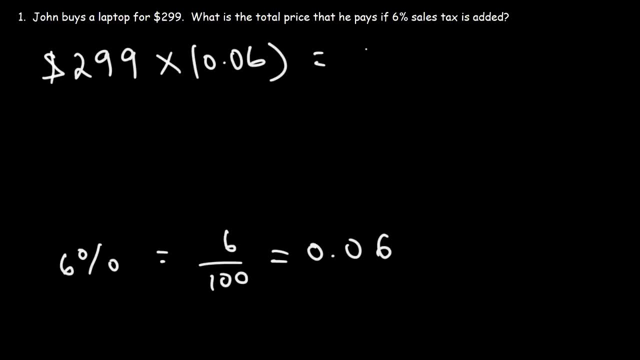 $2.99 times .06 is $17.. So that's 6% of $2.99.. So this is the tax that he pays, plus the price of the laptop, which is $2.99.. So the total price is the sum of those two values, The total. 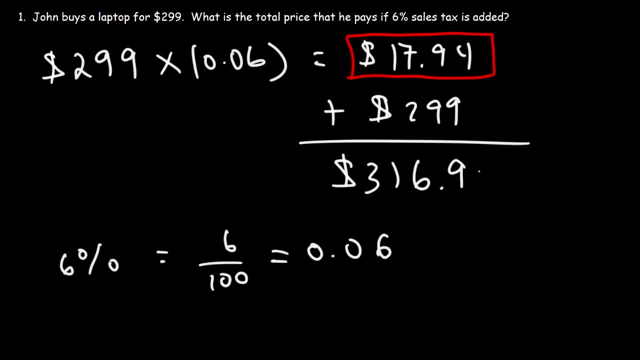 price that he pays is $316.94.. So this is the answer. Now let's look at the next problem. Now, let's look at the next problem. Now, it turns out that there is an easier way to get the same answer. At least it's. 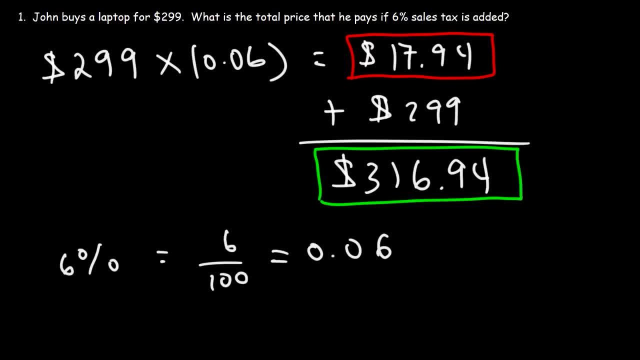 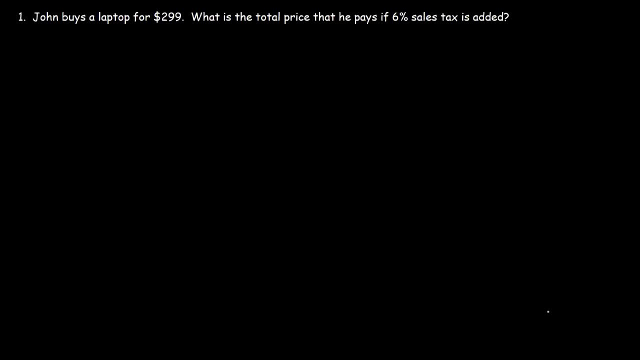 easier, in my opinion, And let me give you the formula, because this formula will help you to solve more complex problems, as you'll see shortly in this video. The new price is equal to the original price multiplied by 1 times- I mean times 1. 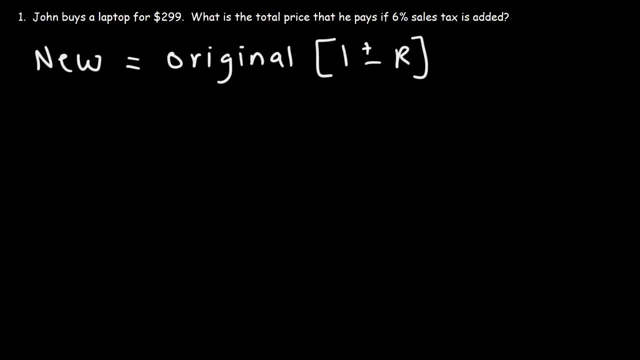 plus the original price. So the new price is equal to the original price multiplied by 1 times. I mean times 1 plus or minus R. Now R would be the percentage when dealing with sales tax. R is positive because you're gonna pay more than the original price. But 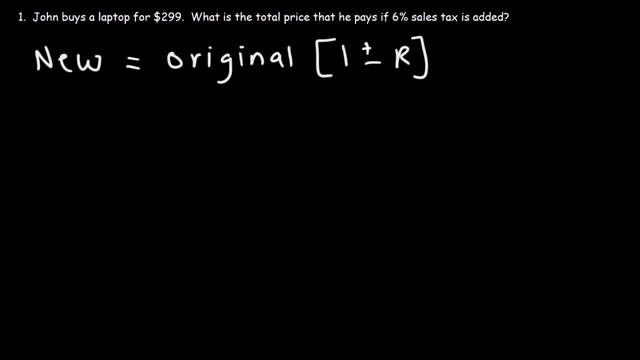 when dealing with discounts, R is gonna have. you can use the minus symbol instead of the plus symbol, because the new price will be less than the original price if you have a percent discount. So in this example, the new price will represent the total price that he's going to pay for the 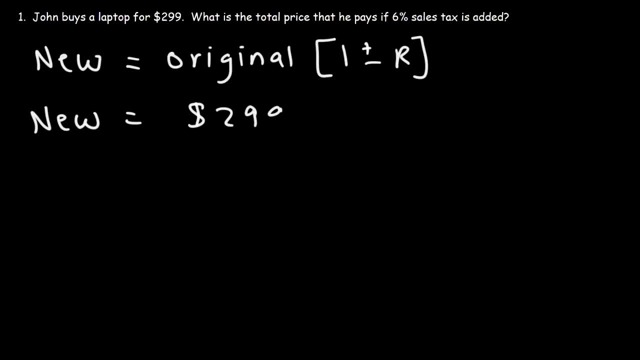 original price represents the price of the laptop, that's 299, and we're going to use the plus symbol, since we're dealing with a sales tax that's going to increase the total price and are is going to be the decimal form of the percentage. six percent is basically .06, so all we need to do is multiply 299 by. 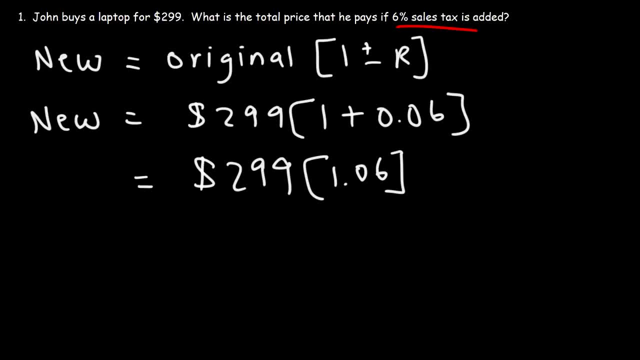 1.06. now, just for you to understand why this works: 299 times one gives you the original price. 299 times .06 gives you that six percent sales tax that he pays in addition to the original price of the laptop, and so that's why we're going to get the same answer. so 299 times 1.06 is 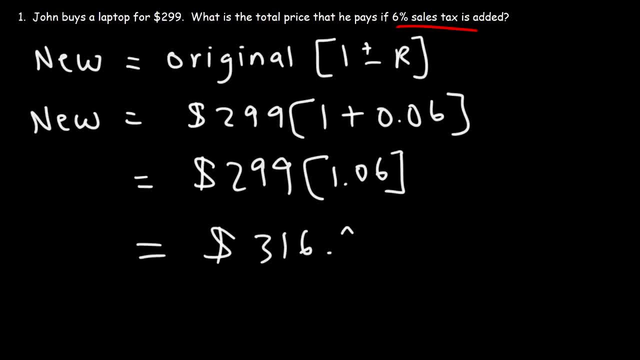 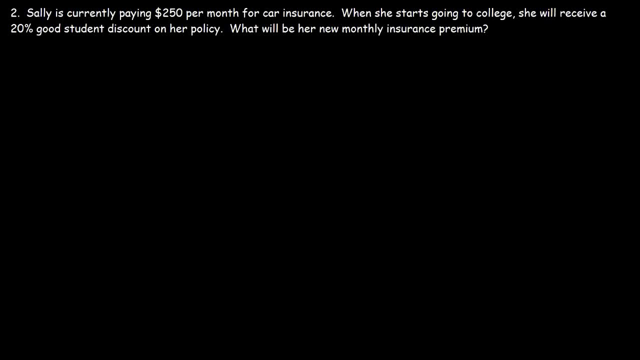 three hundred sixteen dollars and ninety four cents. I believe this method is a lot easier. now let's move on to the next problem. sally is currently paying two hundred fifty dollars per month for car insurance. when she starts going to college she will receive a twenty percent good student discount on her policy. 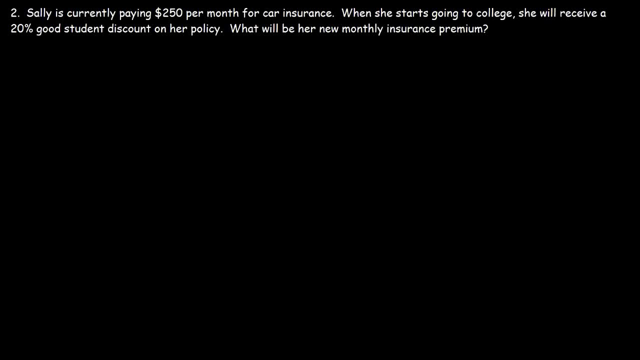 what will be her new monthly insurance premium. so in this case we're dealing with a percent discount, so let's use the same formula. so the new price is equal to the original price multiplied by 1 plus or minus r. So the original price her insurance premiums is $250 per month. 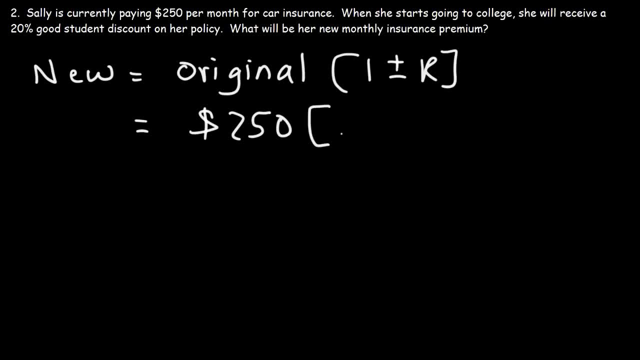 Now she's going to receive a discount, So should we use positive R or negative R? We're going to use negative R because the premiums will decrease after the discount is applied, So it's going to be 1 minus. Now what is 20% as a decimal? 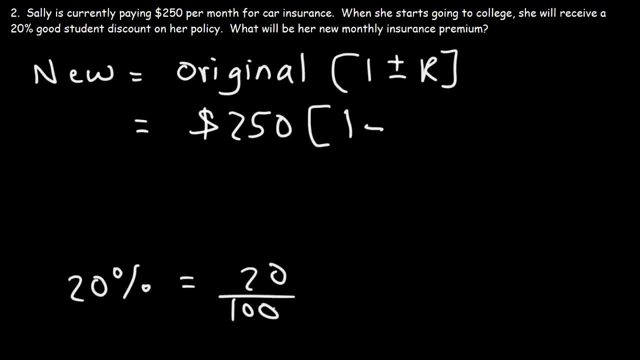 Well, 20% is 20 divided by 100, which is basically 0.20 or 0.2.. 1 minus 0.20 is 0.80.. So she's going to be paying 80% of her original premium, which was $250 per month. 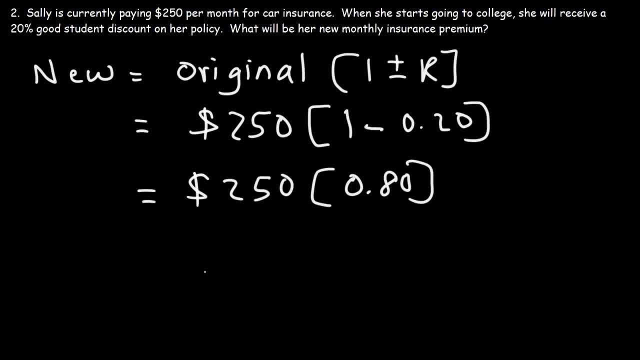 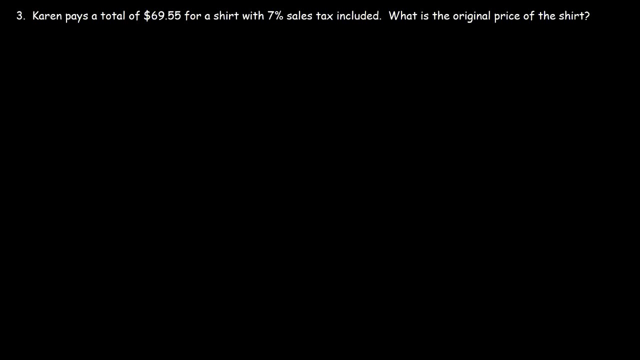 250 times 0.8, that's 200.. So this is going to be her new monthly premium after the 20% discount has been applied. That's the answer Number three. Karen pays a total of $69.55 for a shirt, with 7% sales tax included. 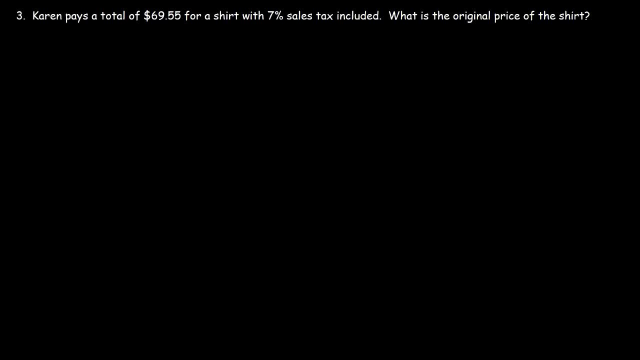 What is the original price of the shirt? Now, in this case, it's going to be very helpful To use that formula. Without the formula, it's going to be difficult to work backwards, So this is when the formula makes life a lot easier. 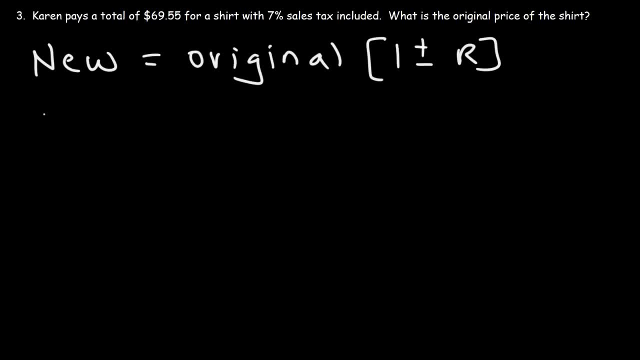 So we have the new price, which is the total price after the tax has been added, And that's $69.55.. We're trying to calculate the original price, so we're going to call it X And we're dealing with sales tax, so that's going to increase the original price. 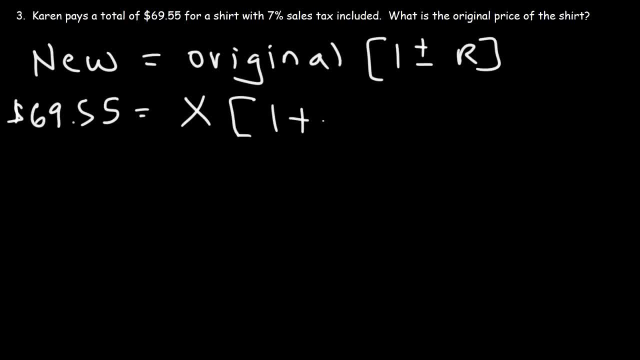 So we're going to call it X, So we're going to use positive R. 7% is 7 divided by 100, which is 0.07.. So we have: 69.55 is equal to 1.07X. 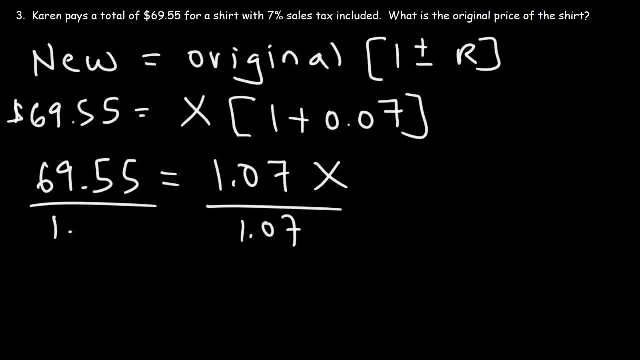 So we need to divide both sides by 1.07.. So let's cancel these two numbers. 69.55 divided by 1.07 gives us $65.. So this is the original price of the shirt. So that's it for this problem. Number four: Gerald buys a car worth $25,000.. The car depreciates by 15% during the first year and then by 10% during the second year. What is the value of Gerald's car after owning it for two years? 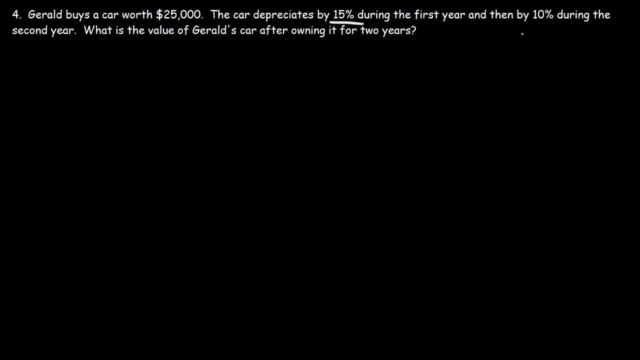 Now we can't combine 15% and 10% and say that his car is going to decrease by 25% over two years. It doesn't work that way. We need to do this one step at a time. So first we need to decrease the car value by 15%. 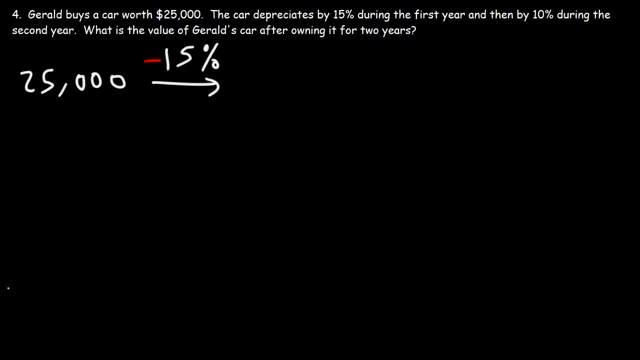 So this would be the same as solving a percent discount. So we could use the formula: The new value is equal to the original value times 1 plus or minus R, So the original value is 25,000.. Since this is basically a percent decrease, we're going to use the negative sign. 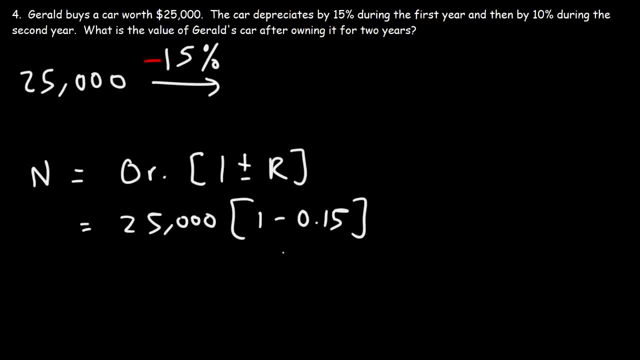 15 divided by 100 is 0.15.. So this is going to be 25,000 times 0.85.. So if we're decreasing 25,000 by 15%, we're basically calculating 85% of 25,000.. 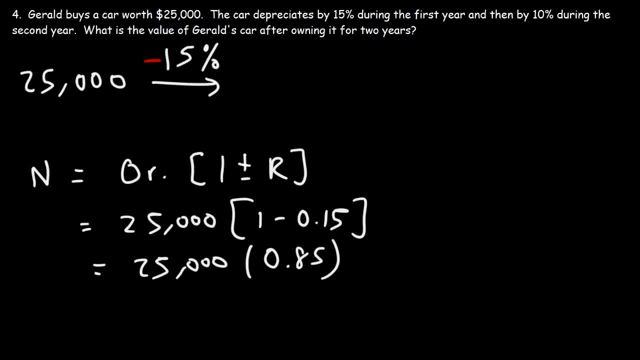 Because 100% represents the whole 25,000.. So 85% of 25,000, or 25,000 times 0.85, that's 21,250.. So that's going to be the new value.